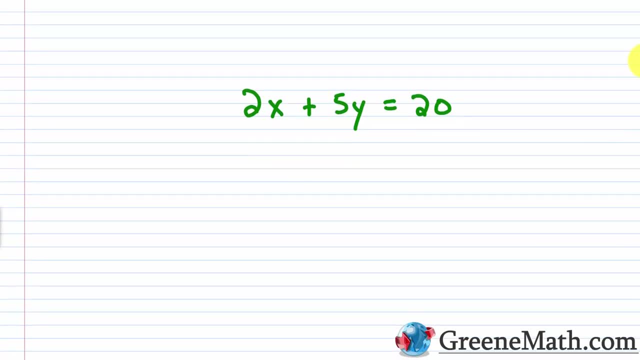 if I wanted to just solve for x, what would I do? Well, if I want to isolate this guy, the first thing I always want to do is isolate the variable term that contains the variable that I'm trying to isolate. So I would start by just isolating the 2x. So to do that, I would subtract 5y away from. 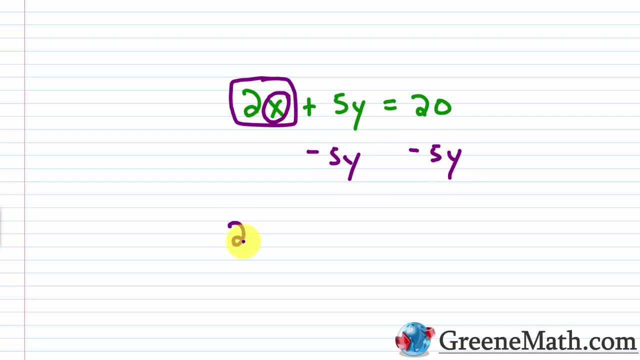 each side of the equation, So I would have just 2x on the left. I know that this would cancel over here, So this equals: now I'll have my minus 5y and then plus my 20.. Now how can I get x by itself? 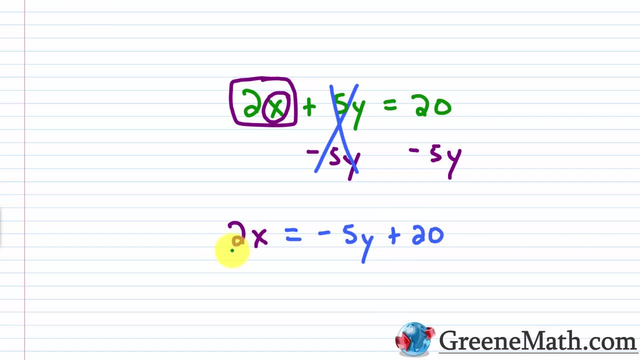 Well, I just have the 2, that's multiplying x. So no change here. I just divide both sides of the equation by 2.. But now over here I'm dividing this whole expression. here I have my negative 5y plus 20.. The whole thing's divided by 2.. And let me scroll down and get a little room going. 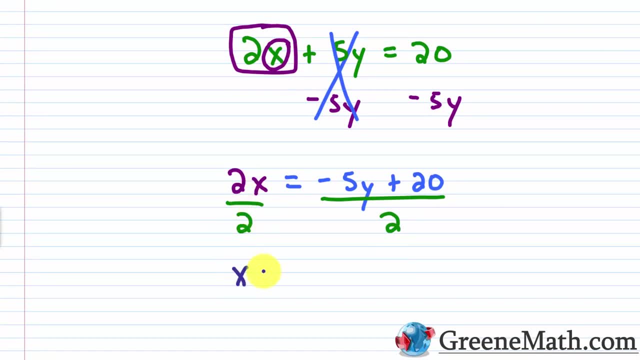 So over here, 2 over 2 is 1.. So I just have x And this is equal to. you have your negative 5y plus 20 over 2.. Now there's different ways to write that. You could split that up as: 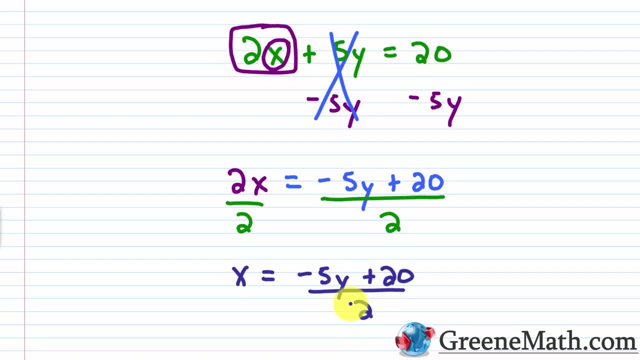 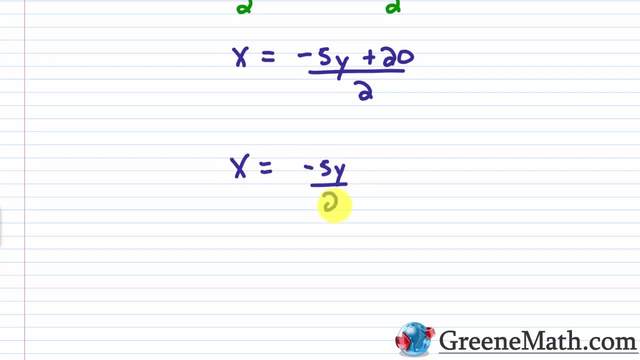 negative 5y over 2 plus 20 over 2.. So I could also say: x is equal to negative 5y over 2 plus 20 over 2.. And, of course, 20 over 2 is 10.. So you could also write it like this: 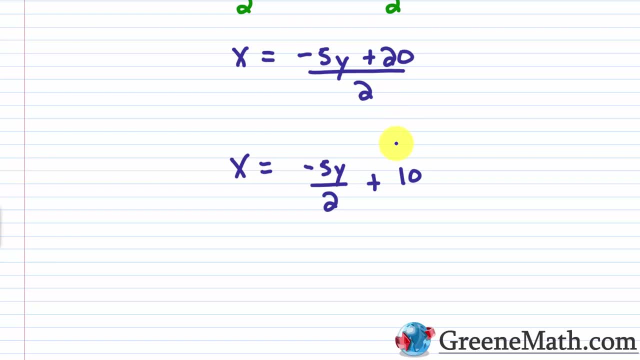 Either answer is acceptable. okay, But I'm just showing you that you can write things in terms of 1 and 2.. So I'm just showing you that you can write things in terms of 1 and 2.. So I'm just. 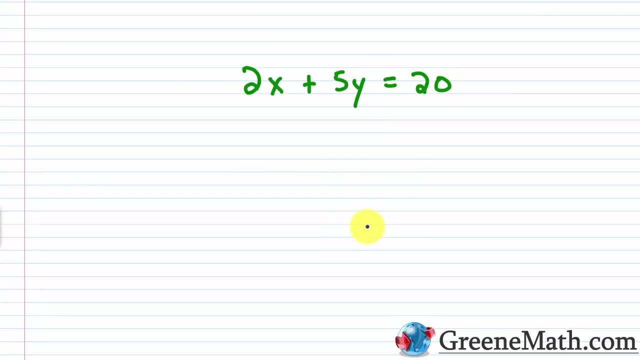 one variable. So I could say x equals something. I can also solve this equation for y. So if I want to solve for y again, the first thing I want to do is isolate the variable term with y involved. So because 2x is being added to this 5y, I just subtract 2x away from each side of. 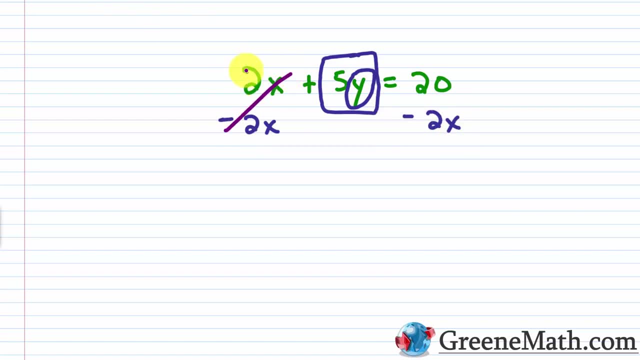 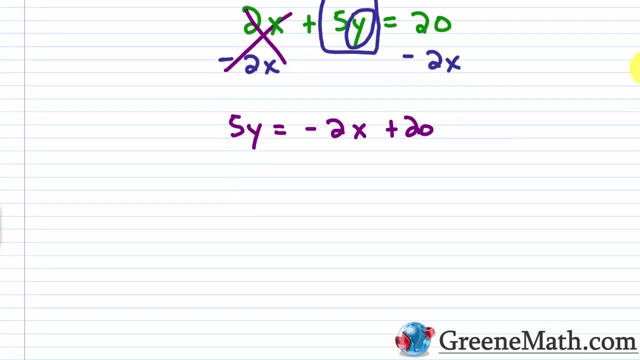 the equation Very, very easy. This is going to cancel. We would have: 5y is equal to you, have your negative 2x and then plus your 20.. And, of course, to get y by itself. I'm just going to. 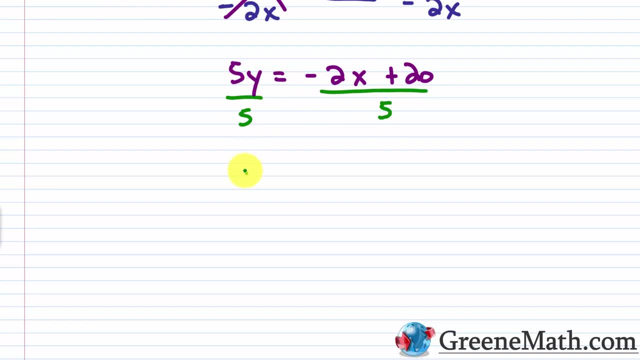 divide both sides of the equation by 5. And so you'd have: y is equal to. you have your negative 2x plus 20 over 5. And again you could write that differently. if you want, You can split that up and. 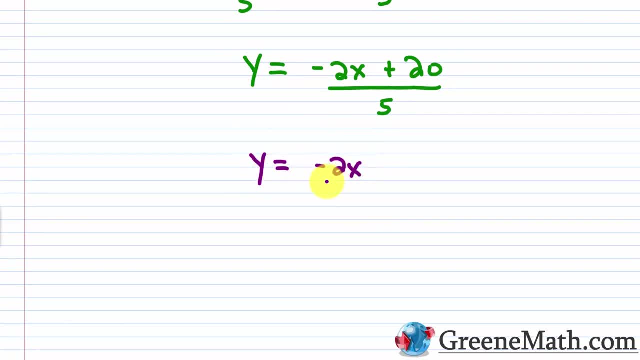 say this is: y is equal to negative 2x over 5 plus 20 over 5.. And 20 over 5 is just 4.. So either way you want to write it, both these answers would be acceptable. We're just showing you that you can. 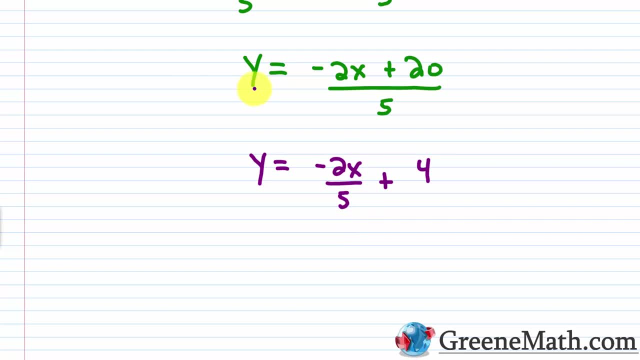 solve for one of the variables, right? So if you want to solve for one of the variables, you can do that. So now this equation is in terms of y: y equals some expression. before we looked at x equals some expression. So when you get more than one unique variable involved, you're not. 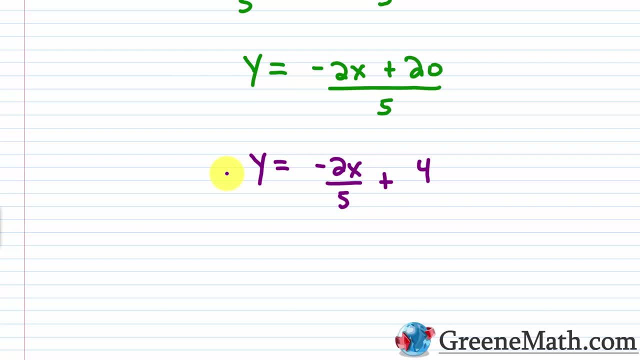 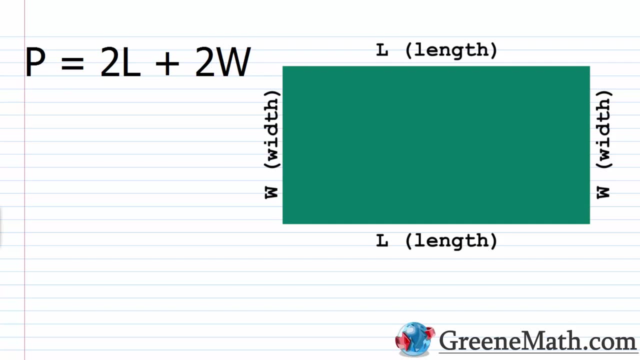 going to have a variable equals some number. You're going to have a variable equals some expression. So normally when we talk about solving literal equations, we're talking about taking a formula and putting it in terms of one of the variables. So this is very useful when we 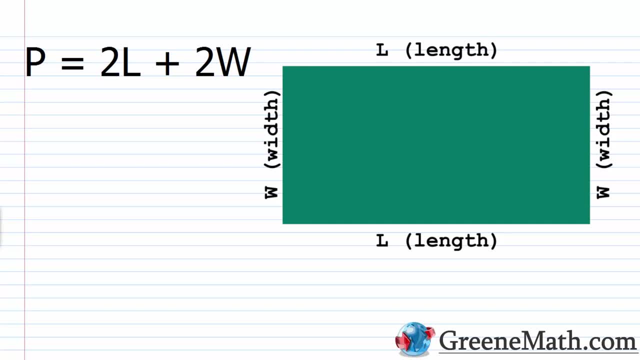 talk about solving word problems. So we're just going to go through a few typical problems that you would see And basically we just need to understand how to solve something for a specified variable. So the first formula we're going to look at is for the perimeter of a rectangle. 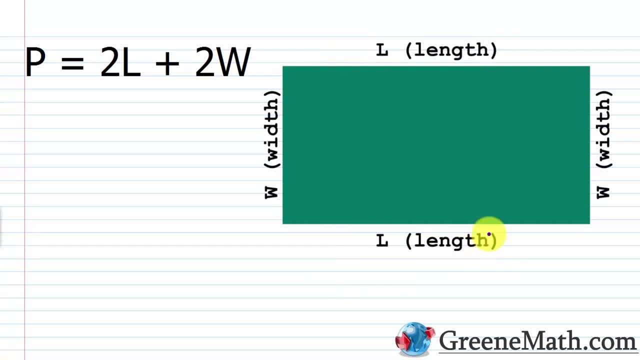 So if you have a rectangle, you have a length here and a length here, So on the top and the bottom, And then on the sides, you have your width right. So length is labeled with L, width is labeled with W. okay, So the perimeter or the distance around a rectangle. 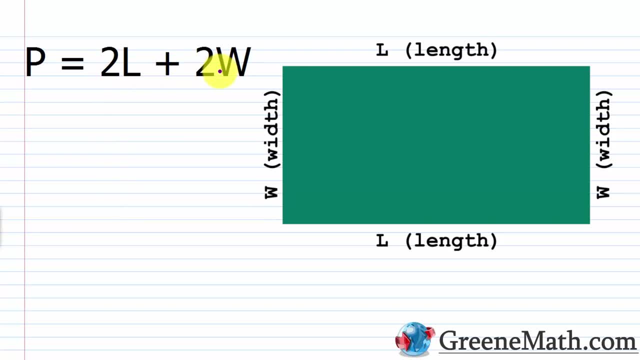 is given as two times the length plus two times the width. okay, So what we want to do here is just solve for W and then also solve for L. Right now you'll notice that it's solved for P, or put in terms of P, because P is isolated on one side of the equation. right You have, P equals some. 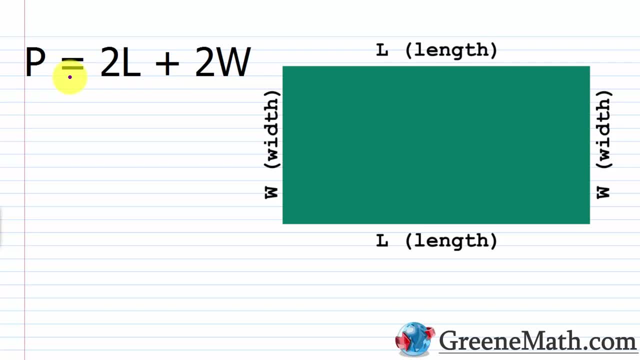 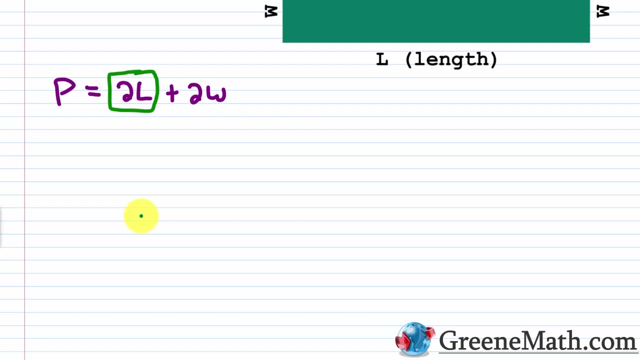 expression. In this case that expression is 2L plus 2W. All right, So to solve for L, let me just rewrite: P equals 2L plus 2W, And if I want to solve for 2L again, I just want to start by isolating the 2L right. Always start by isolating the variable. 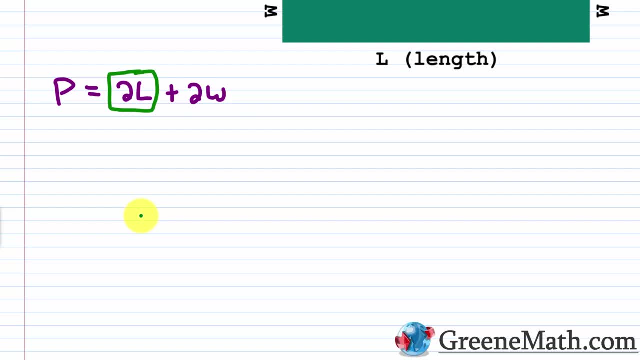 term which contains the variable you want to isolate. So all I need to do is subtract 2W away from each side of the equation. So I'm going to have that P minus 2W is equal to 2L. 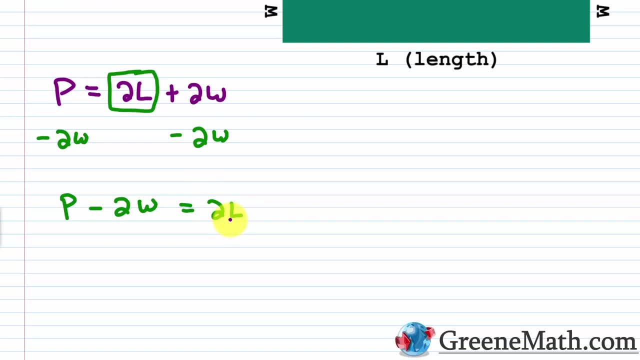 And if I want to isolate L there, what's being done to it? It's being multiplied by 2.. So just divide both sides of the equation by 2. And I'm going to flip this around. So 2s cancel there. 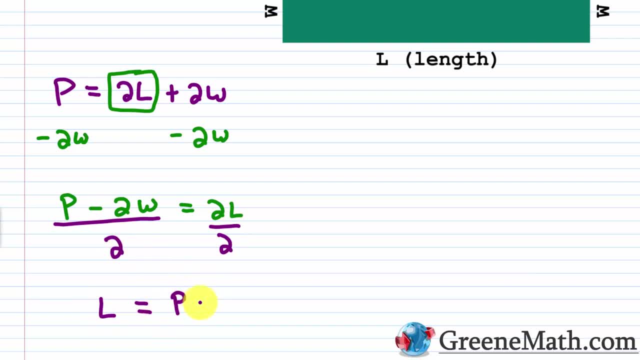 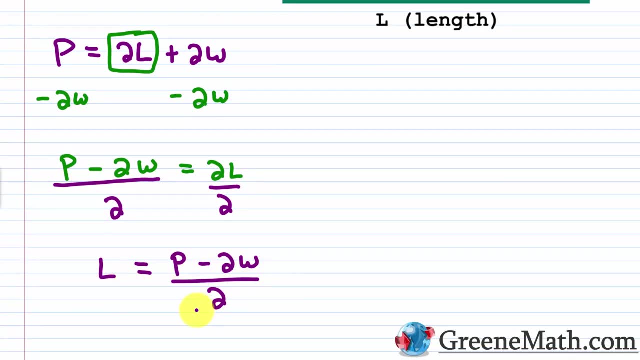 You get: L is equal to P minus 2W over 2.. Okay, So this is in terms of L. now. So if I wanted to put this in terms of W, we'd use the same thought process. So I want to begin by isolating the term with the W involved. 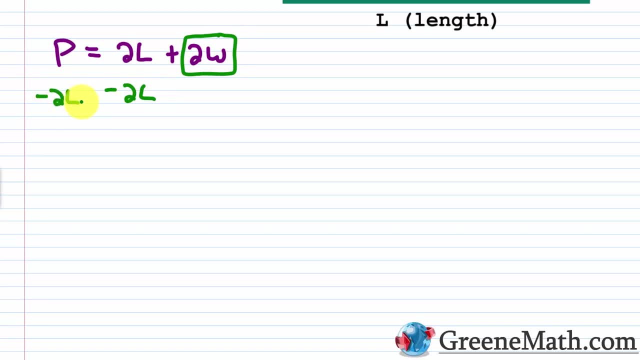 So to do that, I would just subtract 2L away from each side of the equation, So I would have that P minus 2L is equal to 2W. And again, to isolate W, I just divide both sides of the equation by 2.. Okay, Very, very easy, 2 over. 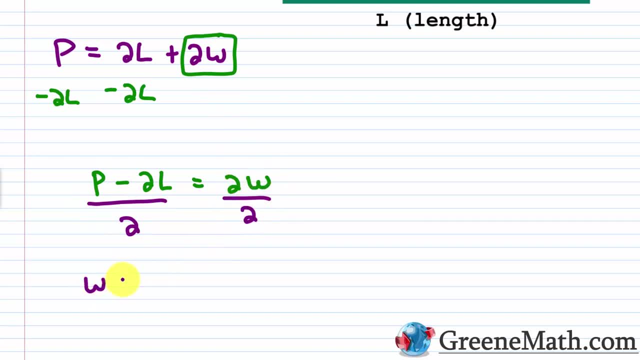 2 is 1.. So you get W is equal to, So W is equal to. You get P minus 2L over 2.. And all I'm doing here is I'm just switching the variable to the left. That's perfectly legal, right, If I wrote. 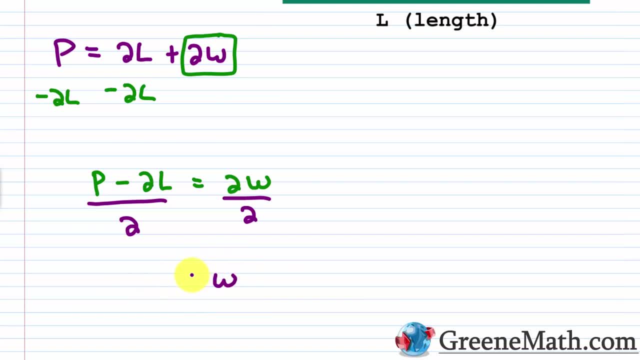 this here as W on the right and this is equal to P minus 2L over 2, I can switch this around and say this is W is equal to P minus 2L over 2.. Okay, It's the same thing. I just like my variable on. 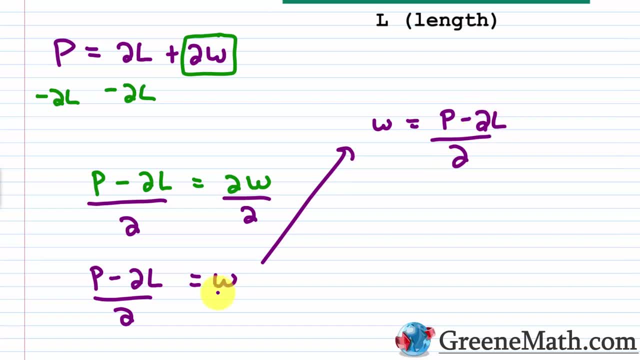 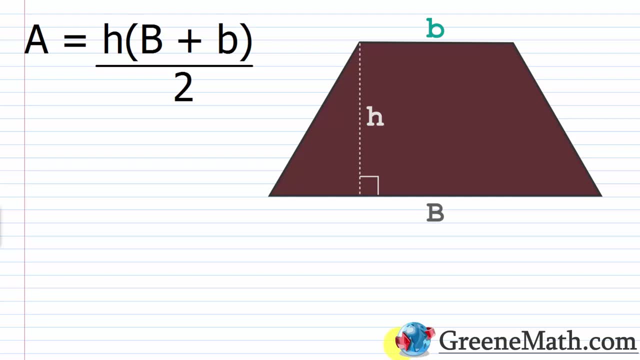 the left. I don't like it on the right, but you can write it either way. They're both acceptable. All right, Let's take a look at another formula from geometry. So we have the area of a trapezoid. 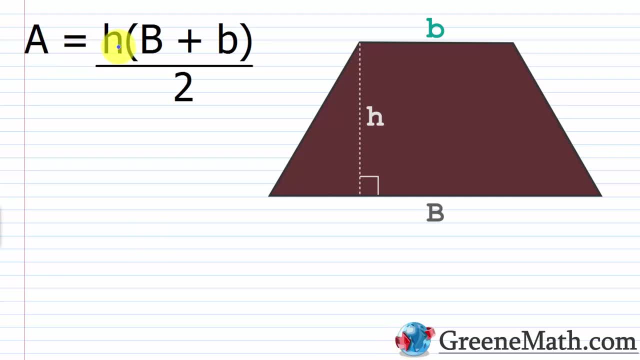 here. So A, which stands for area, is equal to H, which stands for height. That's this guy right here Times the quantity. You have an uppercase B which is down here, That's the lower base. Then plus a lowercase B which is up here, That's your upper base. So then we divide this by 2.. So 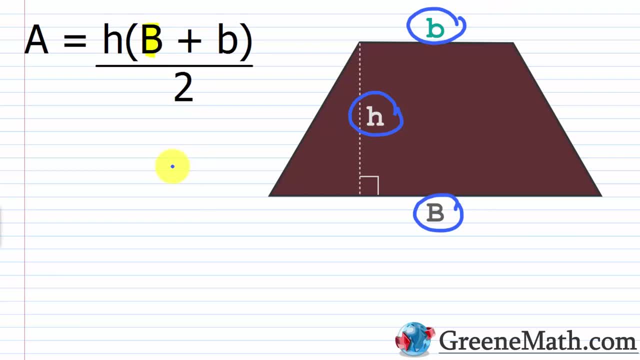 what if I wanted to solve this guy for uppercase B? What could I do? Well, remember, you want to isolate the variable term with that involved first. Right now it's wrapped inside of a set of parentheses, So one thing I could do is just remove the parentheses with my distributive. 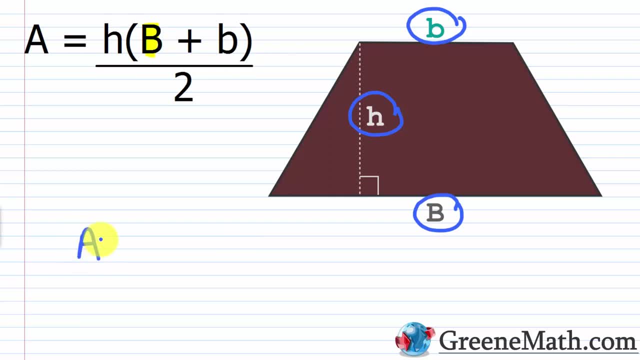 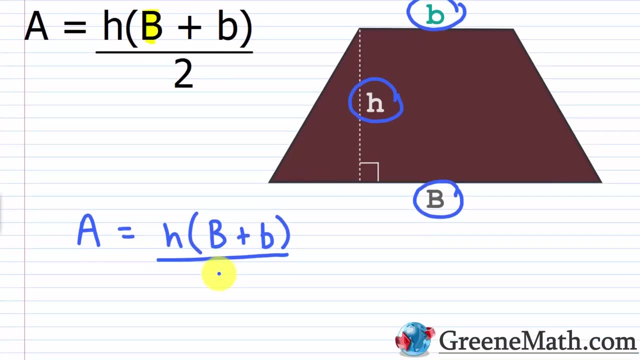 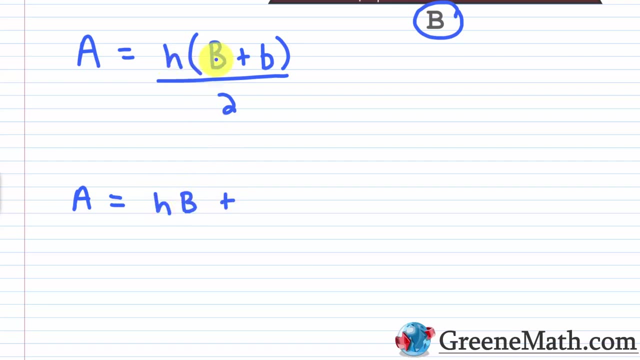 property to kind of get things started. So we would have: A is equal to. You have H multiplied by again uppercase B plus lowercase B, and this is over 2.. So I have A is equal to H times uppercase B, is H times uppercase B. Then plus H times lowercase B is H times lowercase B. 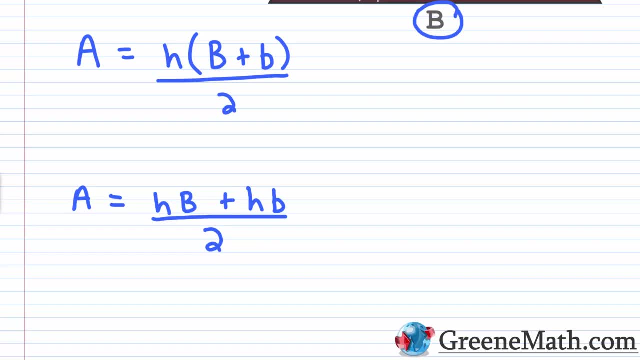 and this is over 2.. Now, if I want to isolate again this term here to start, what I'm going to do is just clear my denominator. I can easily do that by multiplying both sides of the equation by 2.. So this would cancel. Let me kind of go up here. 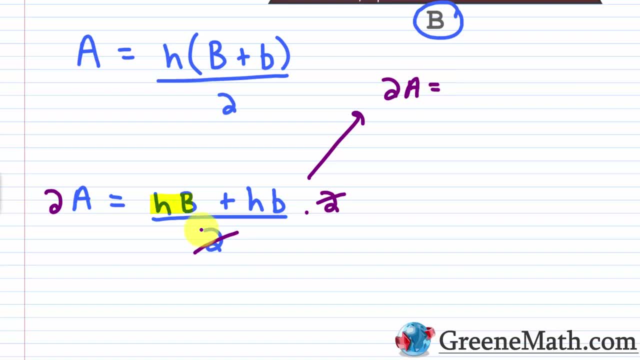 I would have. 2A is equal to. you would have H times uppercase B plus H times lowercase B. Okay, So what do I do from here? Well, I want to isolate again this term right here, because it's got my uppercase B involved. 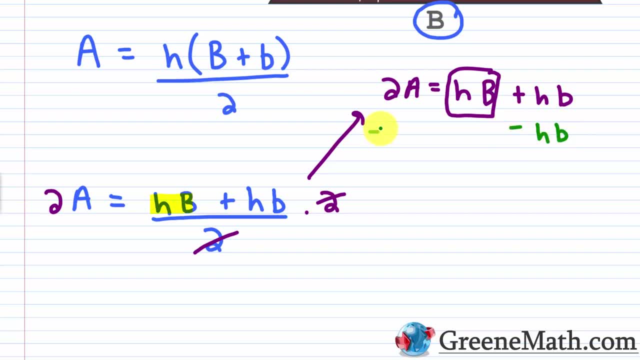 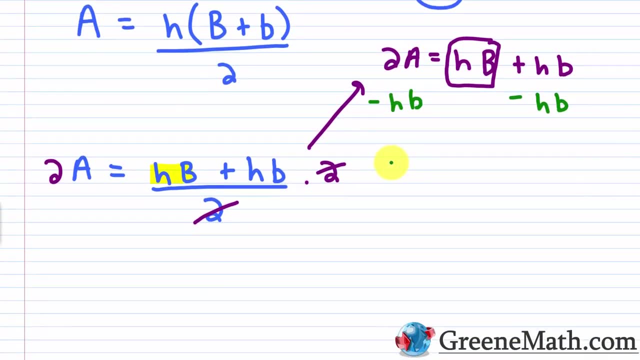 So all I'm going to do is just subtract H times lowercase B away from each side of the equation, And so let me kind of scroll down and get some room going. I'm going to have: 2A minus H times lowercase B is equal to H times uppercase B. 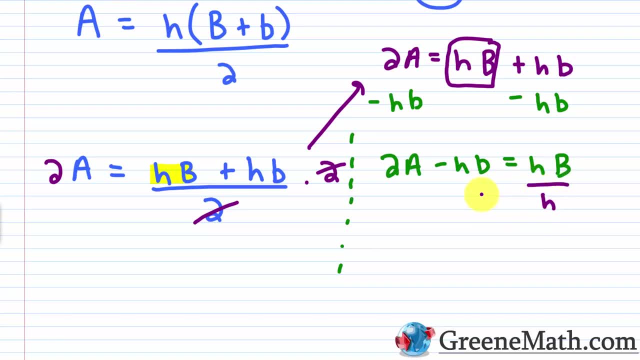 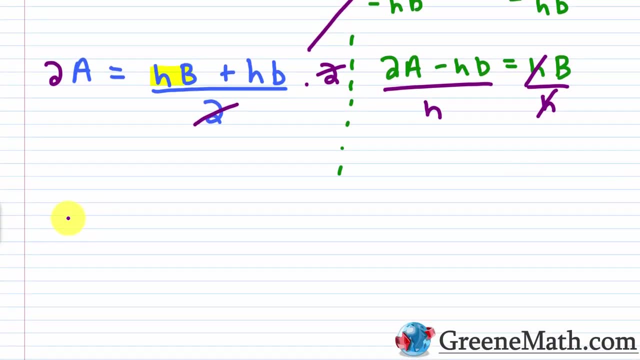 So to get uppercase B by itself, I'm just going to divide both sides of the equation by H and this would cancel, So let me write my answer over here so it's out of the way I have. uppercase B is equal to you. have 2A minus H times lowercase B over H. Okay, 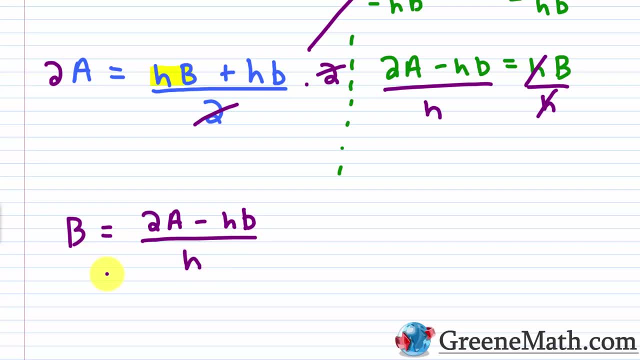 So that's just solving. Let's do this for uppercase B. If you wanted to solve it for lowercase B or you wanted to solve it for H, you would go through the same thought process. So let's go ahead and solve this for H. Let's erase everything. 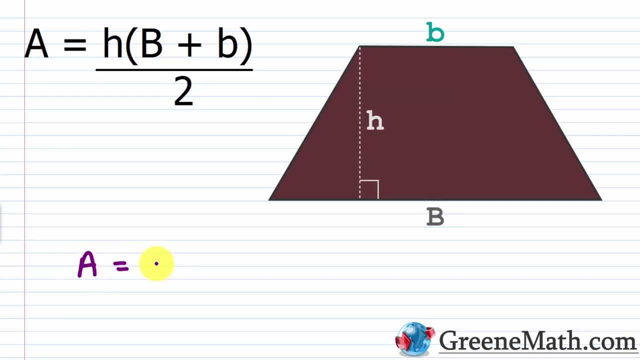 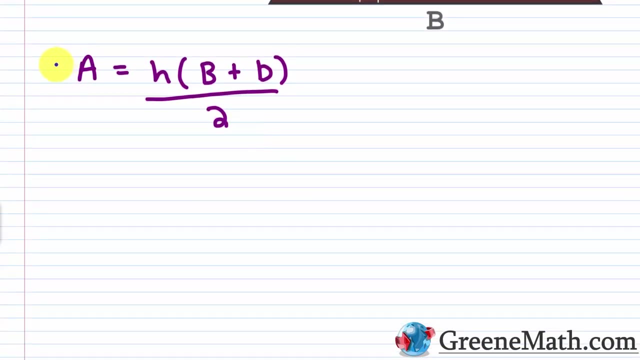 So again, we'll rewrite this formula down here. Area or A is equal to. you have H times a quantity, uppercase B plus lowercase B, and this is over 2.. How can I get H by itself? Well, before I go through and use my distributive property, let's just clear the denominator. 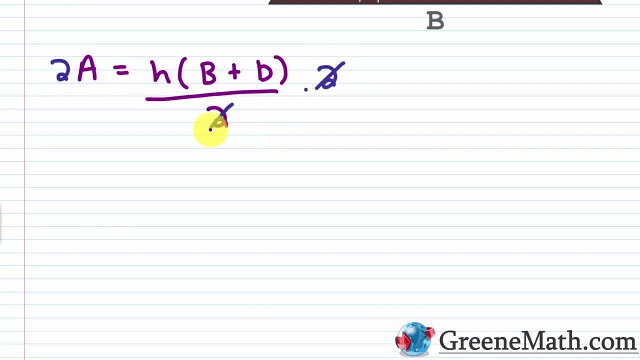 Let's multiply this side by 2.. This side by 2 and this side by 2.. So this cancels. So now I have 2A is equal to. I have H again multiplied by the quantity big B or uppercase B plus small B or lowercase B. Now if I want H by itself, what can I do? 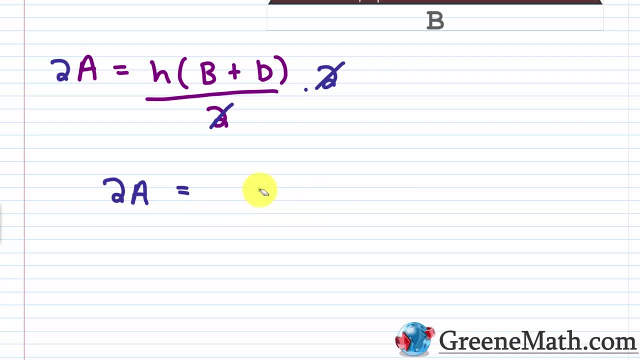 H is being multiplied by something here. Erase this and imagine that you had 4H and you wanted H by itself. You would just divide both sides by 4, right? What's multiplying H? Well, let's go back now. 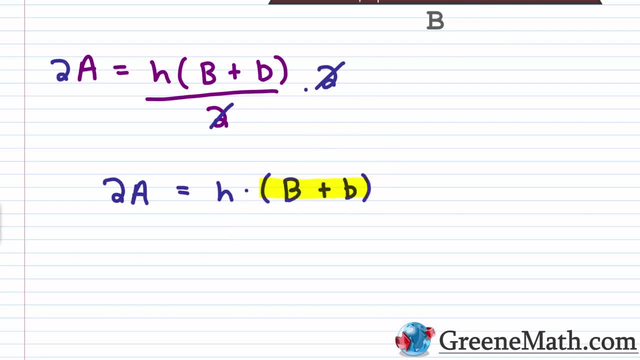 This quantity here is multiplying H, So all I've gotta do is just divide both sides of the equation by that quantity: big B plus little b. so big B plus little b, and I've got my answer. This is gonna cancel. 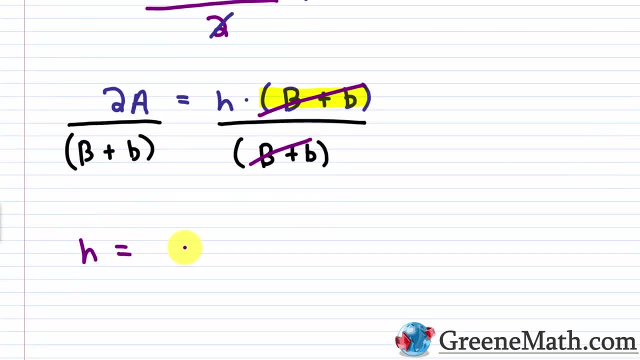 And so what I'm left with here I'm gonna put: H is equal to. you have 2A over bigger B or capital B plus lowercase b. You know that's odd. huh, Let's built in this equation b or smaller b. okay, so now it's in terms of h. all right, let's go ahead and wrap up this problem by. 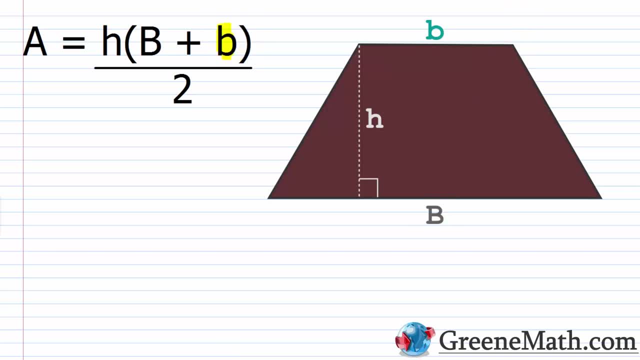 solving the equation for the lowercase b. now and again, the idea is always the same. if i'm solving for the lowercase b, i just want lowercase b on one side of the equation and i want an expression on the other. okay, so very, very easy. so we have that. a is equal to. we've got h multiplied by the. 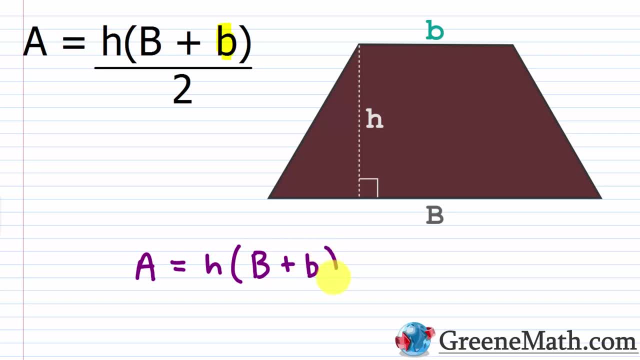 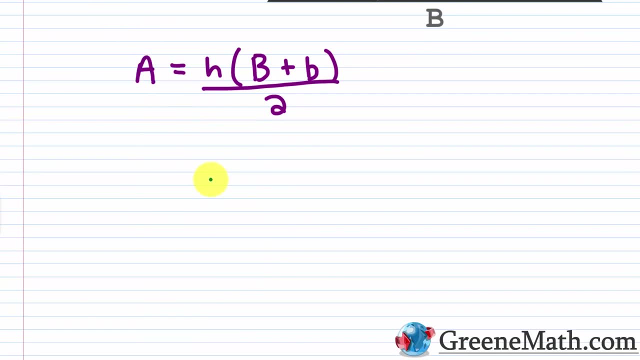 quantity. you've got your uppercase b plus your lowercase b and this is over two, and let's get some room going here now. there's many ways to start this problem. you can start by using your distributive property to remove the parentheses, because ultimately you need to get to that b. 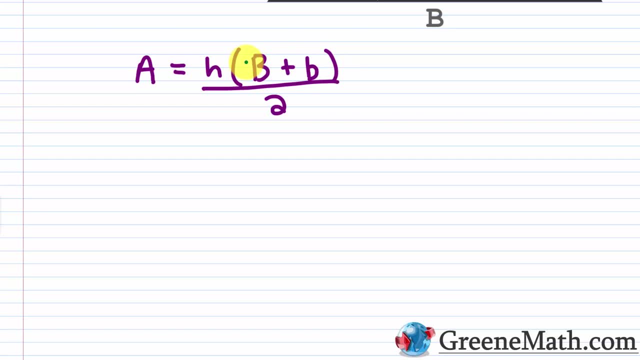 and it's inside of parentheses right now. so that's one thing you can do. another thing you can do is you can clear the denominator first. so we can do that and let's just start by that. so we'll go ahead and cancel this with this and we'll do. 2a is equal to we've got h times the quantity you've. 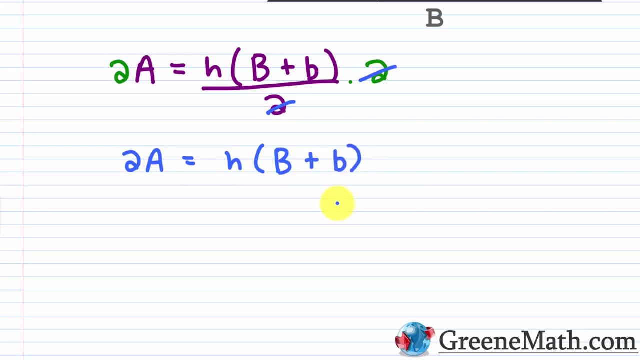 got your uppercase b plus your lowercase b. you've got your uppercase b plus your lowercase b. and you've got your uppercase b plus your lowercase b. now you can use your distributive property to remove parentheses. that's fine. that's one way to do it, or another way and probably a faster way. you can just divide both. 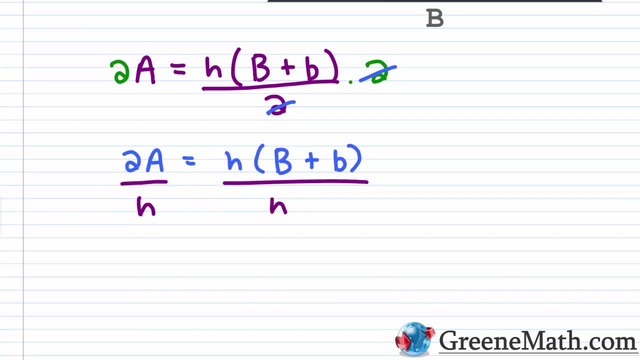 sides of the equation by h. right, because if you divide both sides of the equation by h, then you can go ahead and remove those parentheses. you'll have access to this lowercase b here, so i'll have 2a over h on the left. this is equal to now. i just have the capital letter b plus the lowercase b on. 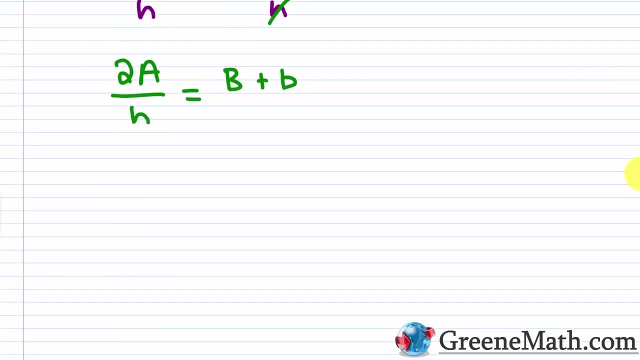 the right. okay, so to solve for the lowercase b now is very, very easy. i just have this capital letter b that's being added to it, so i'm just going to subtract the capital letter b away from each side of the equation, and so i'm going to end up with 2a over h minus the capital letter b, and this is equal to. 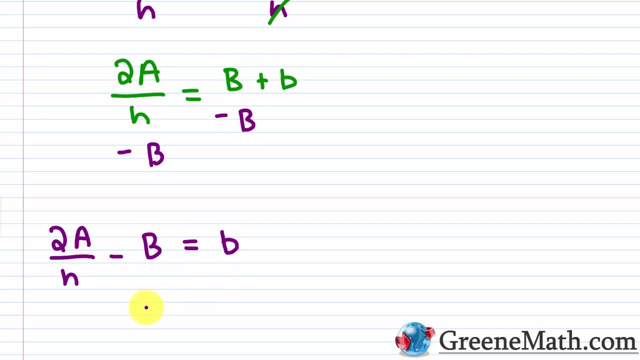 the lowercase b. okay, and if you like the variable on the left, like i do, you can rewrite this. you can say: lowercase b is equal to 2a over h and then minus uppercase b. now you'll notice that we don't have a common denominator here. 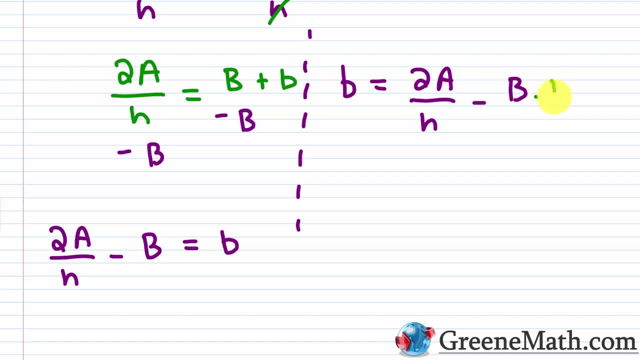 if we want a common denominator, we can get one. we can just multiply this by h over h. if we were to use the distributive property, we would have gotten one. so this is just a matter of personal preference. it's the same answer either way, so i can write this as lowercase b. 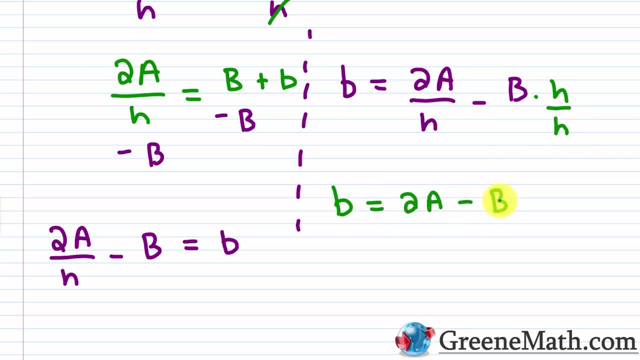 is equal to 2a minus uppercase b times h, all over the common denominator of h, or again it's the same thing. if you say lowercase b is equal to 2a over h minus uppercase b, all right, let's look at some other problems. so suppose i wanted to solve this for. 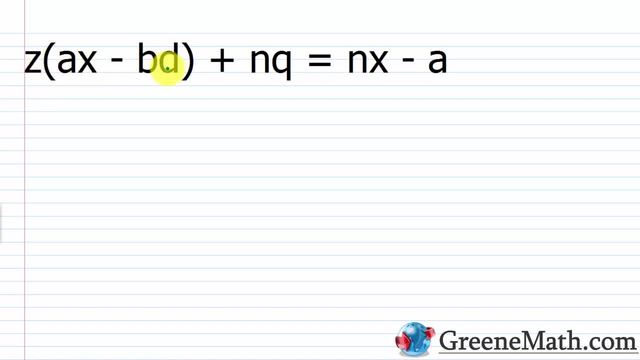 just x. so z times the quantity ax minus bd plus nq equals nx minus a. how can i solve this for x? i have an x here and i have an x here. well, if you get this scenario, you've got to get all the terms with an x involved to one side and everything else to the other. so let's go ahead and distribute this. 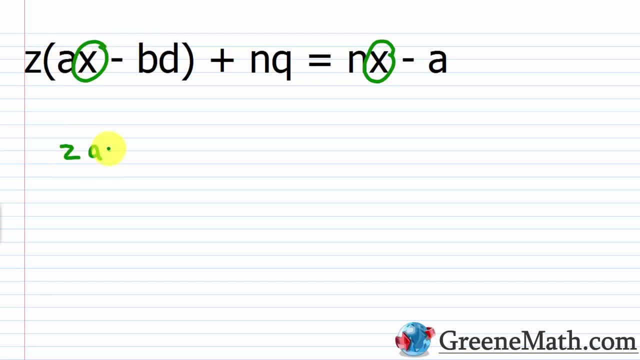 z to each term inside the parentheses. so you would have zax minus zbd, then plus nq, this is equal to nx and then minus a. so i want this term and this term because they each have an x involved on one side of the equation. i want everything else on the 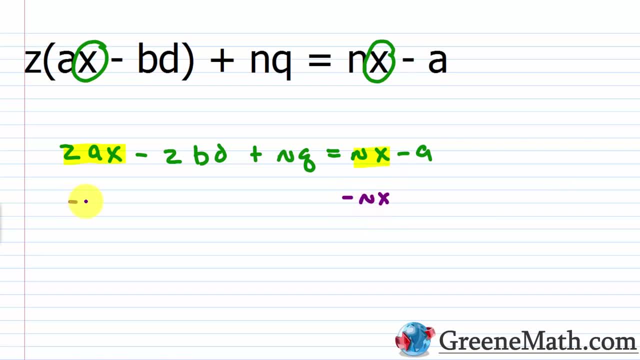 other. so what i'm going to do is i'm going to subtract nx away from each side of the equation and i'm going to add zbd to each side of the equation, and then i'm going to subtract nq away from each side of the equation. 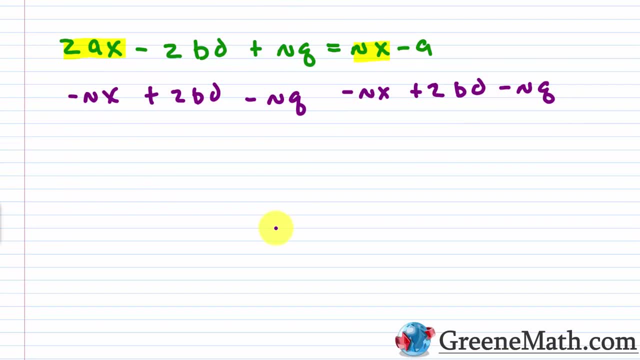 okay. so a lot of stuff on the screen here. let's go through this. so this is gone, i've cancelled it. and this is gone, i've cancelled it. so on the left i'm going to have zax minus nx, then this will be equal to. on the right, this is going to cancel. so i'll just have negative a plus zbd. 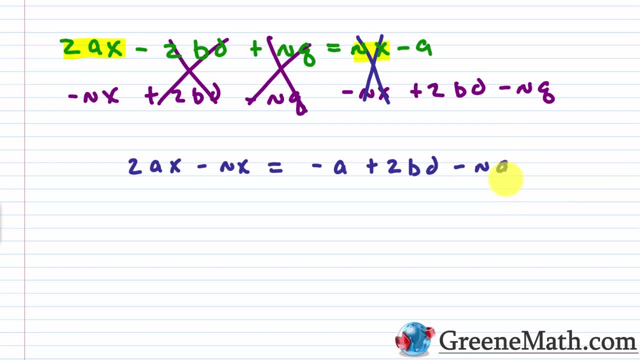 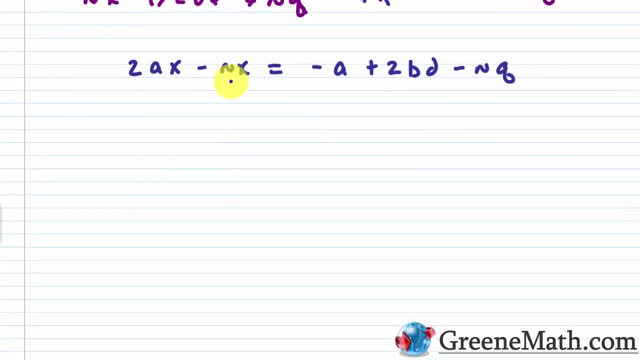 minus nq. let me make that q a little bit better, okay. so how can i solve this for x? a lot of you, if you see this, will be perplexed. what can i do here? well, think about this: if you had something like 6x minus 4x, we know we can combine like terms there, but why can we do that? well, because of 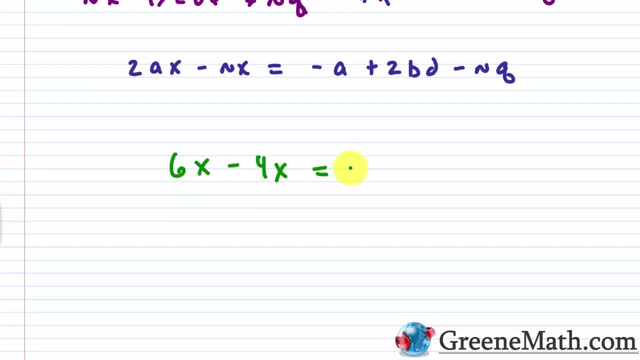 the distributive property, i can pull the x out and i can say: this is 6 minus 4 inside, so this becomes x times 2 or 2 x. if i use the same thought process here, i can pull my x out because it's common to each right. every time every one of our vectors have fake x's in here, so we get 2 times 2. 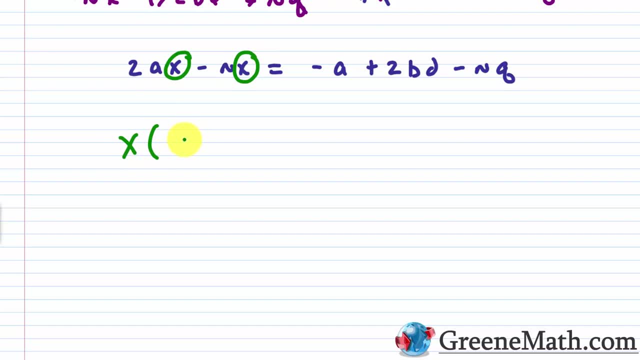 so it's a pretty simple way. if you use the same thought process here, i can pull my x out because it's common to each right. so if I pull that out inside the parentheses I would have ZA minus N. now I can't combine those, but that's okay, you'll see in a minute. I can just divide by that, because that's what's multiplying X. 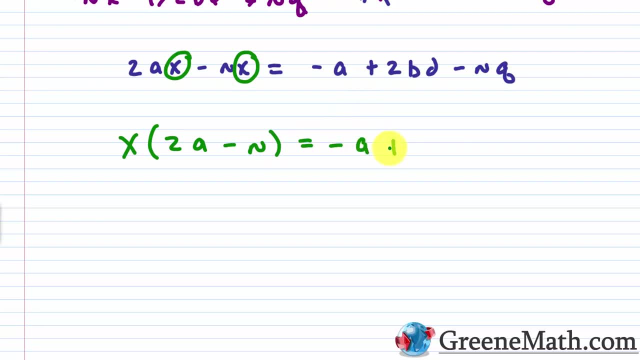 and this is equal to. you have your negative A plus your ZBD, then minus your NQ. now again, this is multiplying X. so it's just like if I had 4X is equal to 20. if 4 is multiplying X, I can divide both sides of the equation by 4 so that X is equal to 5. same thought process here, all I want. 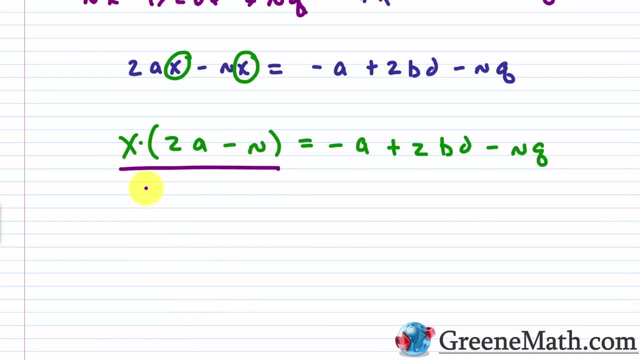 to do is divide both sides of the equation by what's multiplying X. so it's the quantity ZA minus N, and I'm going to divide by that over here as well. so ZA minus N, and it looks messy, but this is what we need to do when we have a lot of variables involved. so I've solved this for X. 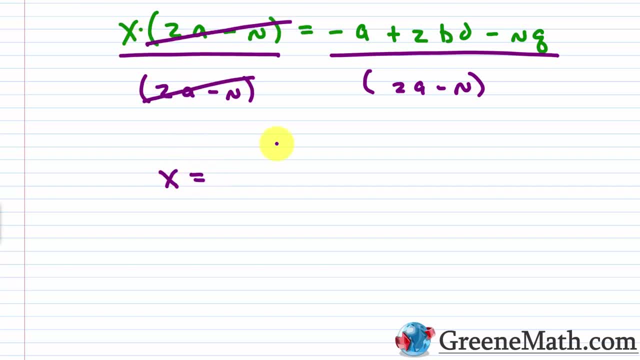 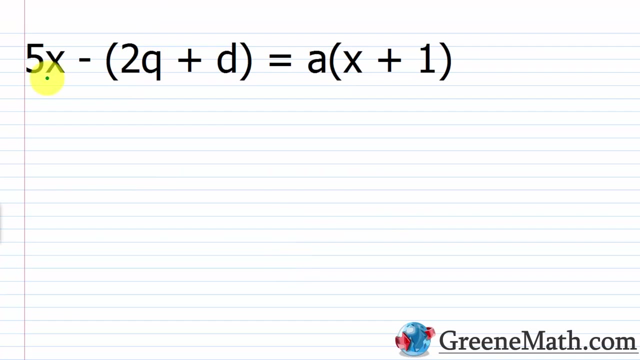 now, because this is going to cancel you. you have X is equal to. you have your negative A plus your ZBD, then minus your NQ over you have your ZA and then minus N. all right, let's go ahead and take a look at another one. so we have 5X minus. 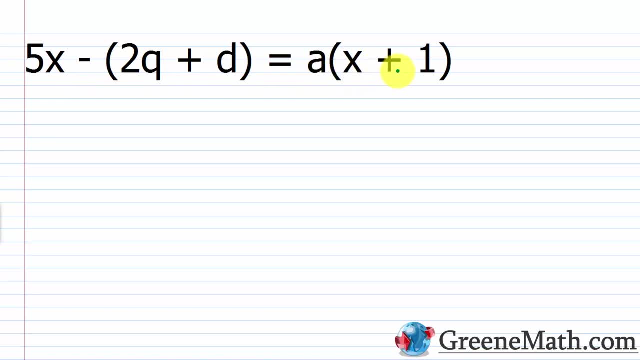 the quantity 2Q plus D is equal to A times the quantity X plus 1, so we want to solve this for X. and again, the idea here is, if I want to solve it for X, I've got to first get all the variable terms with X involved on one side, and every time I do that I'm going to get all the variables. 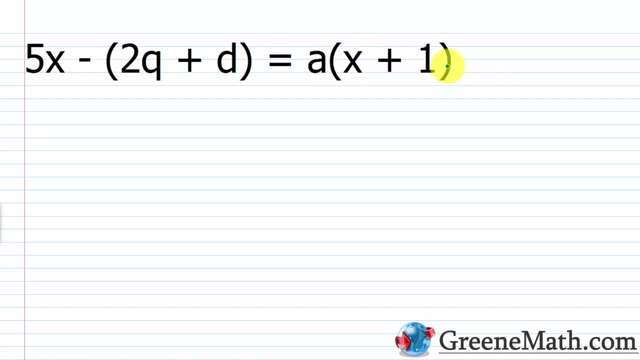 in the other. so because I have an X here wrapped inside of some parentheses, let's go ahead and use our distributive property, get everything simplified. so we have 5X. I have this negative out in front of these parentheses. so again you can think about this as plus negative 1. the negative 1 would. 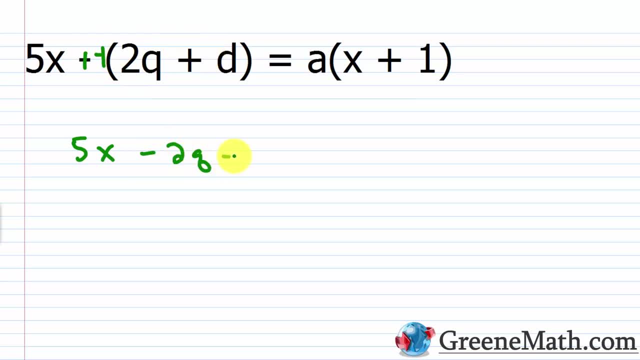 multiply by each term. so you'd have minus 2Q and then minus D and this equals the A is going to multiply by each term, so AX and then plus A. okay, so I want all my again terms with an X involved on one side. so let's go ahead and subtract AX away from each side of the equation and let's add 2Q. 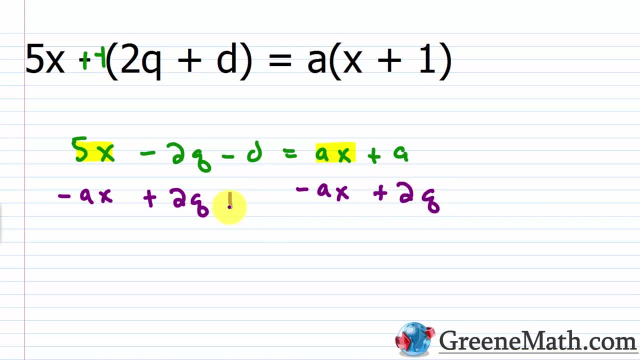 to each side of the equation. and let's add D to each side of the equation, okay. so this would cancel here, this would cancel here and this would cancel here. so on the left-hand side, I've got 5X minus AX, and this is equal to. on the right-hand side, I've got A plus AX minus AX, and this is equal to. 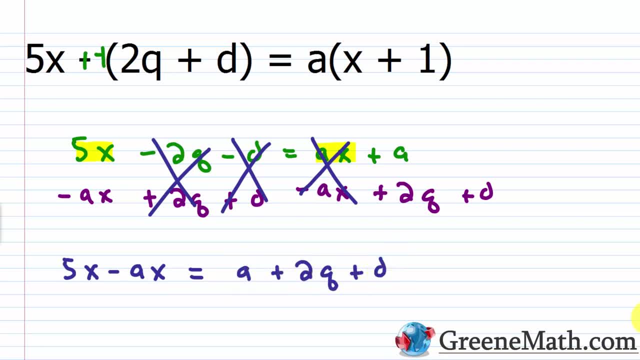 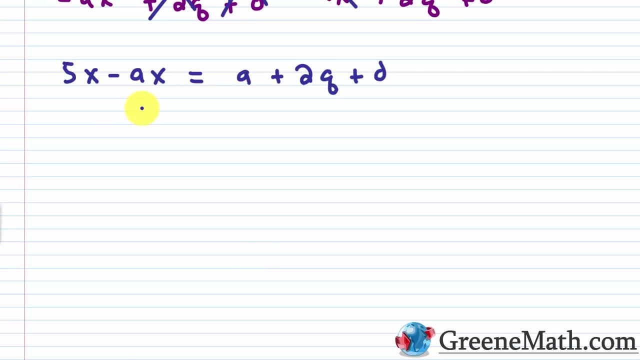 2Q plus D. All right, So now, what do I have here on the left? How can I isolate X? Well, again, I think about the process. I used to combine like terms. If I have 5X minus, let's say 6X. 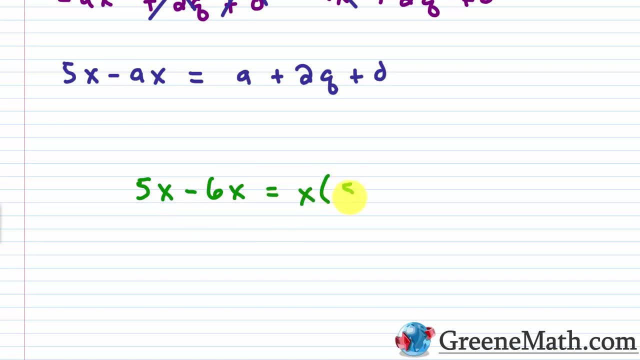 well, I can factor out the X there And inside the parentheses I would have 5 minus 6.. We know 5 minus 6 is negative 1. So this is negative 1X. Well, here I can basically again do the same. 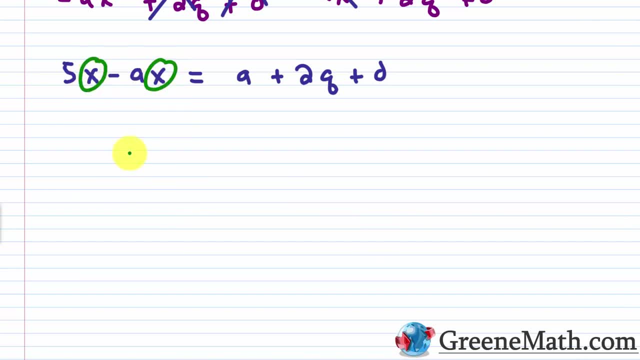 thing. I can factor out the X because it's common to each. So I can have X times the quantity 5 minus A. This is equal to A plus 2Q plus D, Since this quantity 5 minus A is multiplying X. 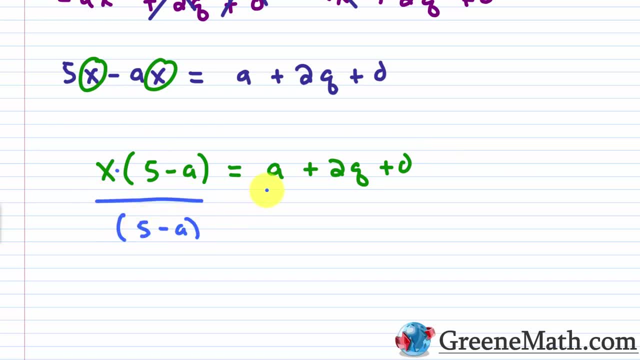 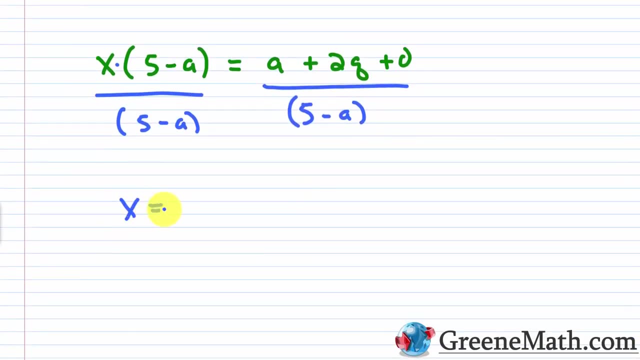 to get X by itself, I just divide both sides by that quantity And I'll have X by itself. So I will have. X is equal to: we'll have A plus 2Q plus D over your 5 minus A.